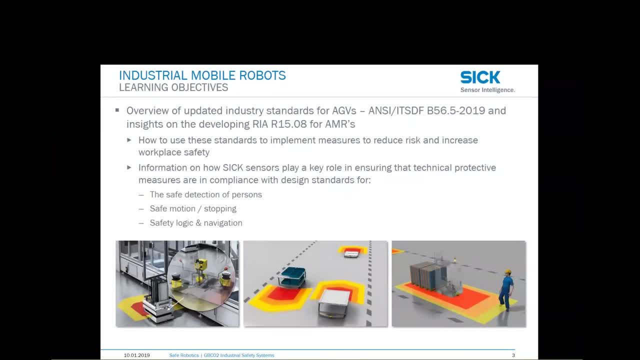 And we're going to update, give you a little update on a few industry standards that provide guidance for the safe design and the construction of these types of vehicles and some of their similarities and some other differences. We'll review some of this background and a couple of different standards. the revised version of the IPSDF B56.5 standard for AGVs. 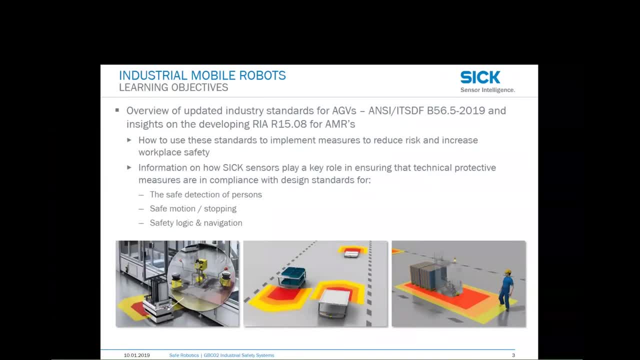 And a developing standard for Autonomous Mobile Robots and the RIA R1508.. The presentation should take about 45-50 minutes and we'll leave some time at the end for questions And, as Lisa mentioned, you can type those questions into the Q&A as it progresses and then we will cover those at the end. 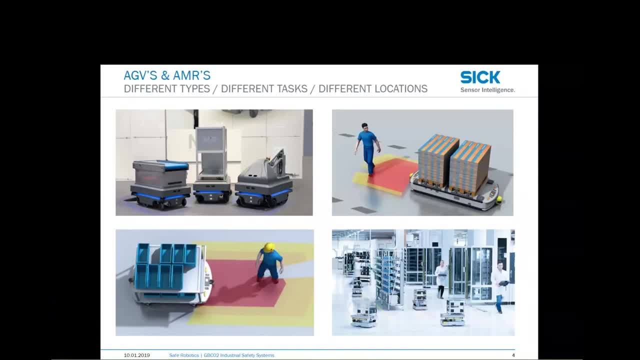 So there's a lot of common technology behind both AGVs and IMRs. However, there are a few key differences that require the application of the guidance that are found in these C-type standards. we're going to discuss a little bit today Each of these mobile platforms. it is imperative that we think about designing, constructing and implementing them safely, And to do that, we need to understand these key differences. 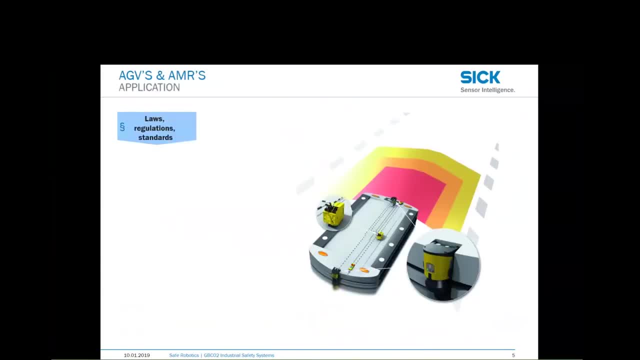 One thing that is common, however, to both AGVs and AMRs is that we'll follow a process of thinking about how to design, construct and implement them safely throughout their life cycle. We talk about the six steps to any safe machine, and it applies certainly to these types of vehicles. 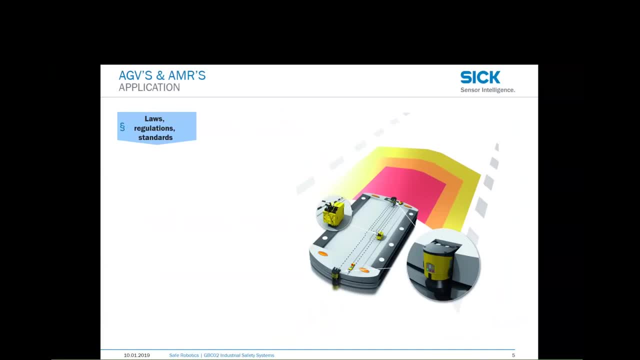 Typically, we have to look to the laws, the regulations and the standards that helps support those laws and regulations and this is where we find our benchmark. This is where we find the target that we're trying to hit when we when we're working on the software. 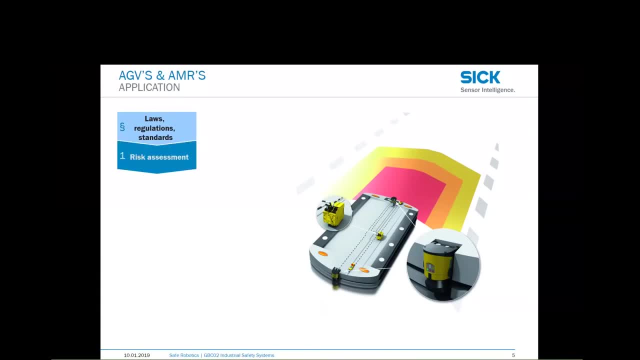 with these types of platforms. once we understand the what we need to do, we're going to conduct a risk assessment to identify all those tasks performed in and around the environment of the of the platform, and it's the affected personnel that may come in contact with the platform as it's moving stationary doing. 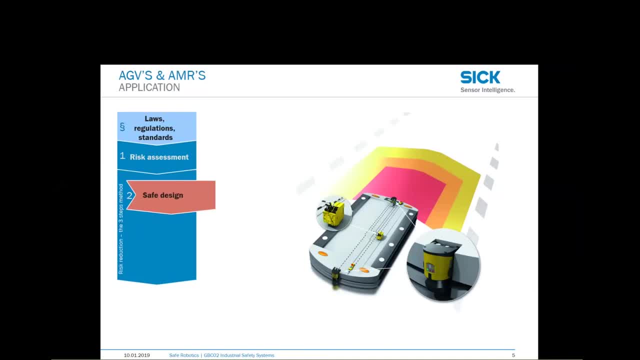 its work. the information from the risk assessment leads us to the risk reduction. how are we going to handle these interactions in a safe way? so we talk about safe design measures, we talk about technical protective measures implementing safety functions to controlling the movement and the hazardous motion and, in the end, we want to inform users of the devices how to. 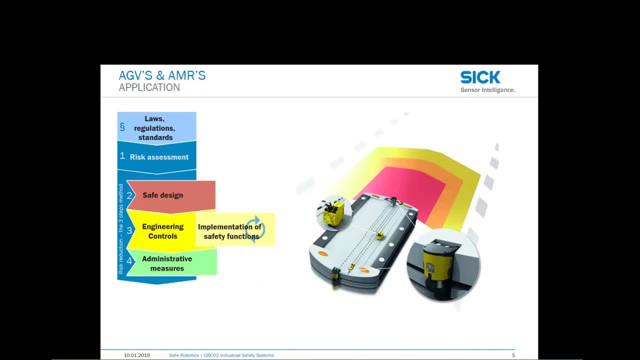 implement them safely and you awareness measures, horns, beacons, signage, training, those types of things that also add to the overall risk reduction of the safe implementation of such platforms. and in the end we want to evaluate to make sure that we've achieved their aims that we set forth in the risk assessment, and then we can place the system or the 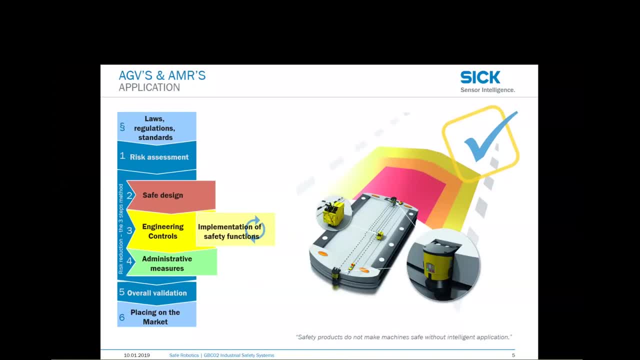 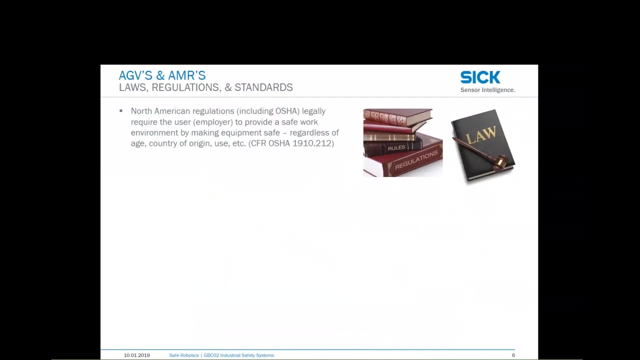 platform on the market and, in and over its lifetime, that we can use it safely in the manner as intended. so let's take a look in North America. you are the laws and regulations, and how do we pull these together to support the use of the standards? that's the way we do. OSHA is our legal framework in North. 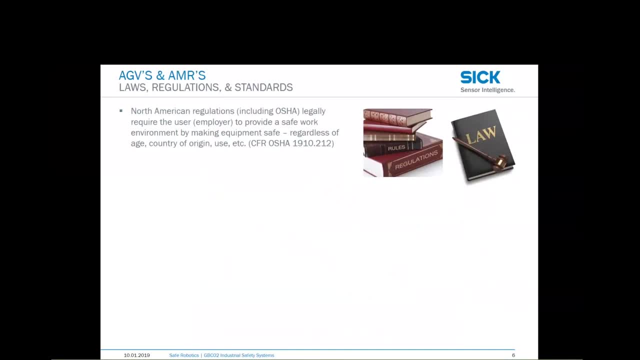 America, specifically in the United States, and we look to the code of federal regulations under 1910 to 12 where we'll find the general duty clause that what's the onus of a safe work environment on the employer right, really the end-users Authorized? we need to find information of how to do this properly and we find that. 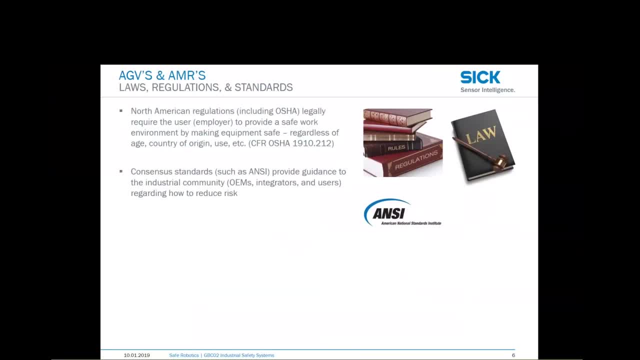 information or the guidance of how to design and and build and construct these, these types of machines, or any machines and platforms, through consensus standards. so we'll talk about a couple these consensus standards today that are both happen to be ANSI standards, some American National Standards Institute, so 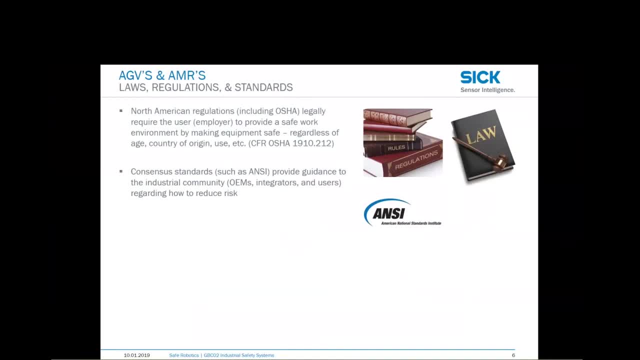 So the developing organizations who have taken the time to organize and develop these standards under the ANSI framework can publish these as ANSI standards. One thing to keep in mind: that the ANSI standards are third-party consensus, They're voluntary standards. They're not cited necessarily by regulatory requirements. 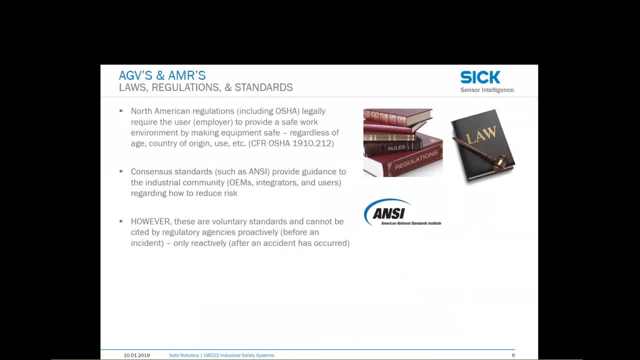 There's no requirement, But they do provide a very well-thought-out, state-of-the-art, industry-accepted methodology for doing this properly And therefore, by complying with the tenets found in these consensus standards, you can go a long way to ensure that you've met the requirements set forth in OSHA. 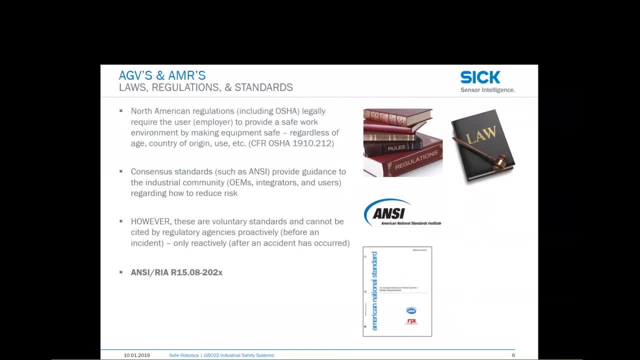 A couple of standards we're going to talk about today: a new developing ANSI RIA standard, the RFI. This is R1508.. It is under development. It's for industrial mobile robot safety, so we'll talk about what's new in that standard. 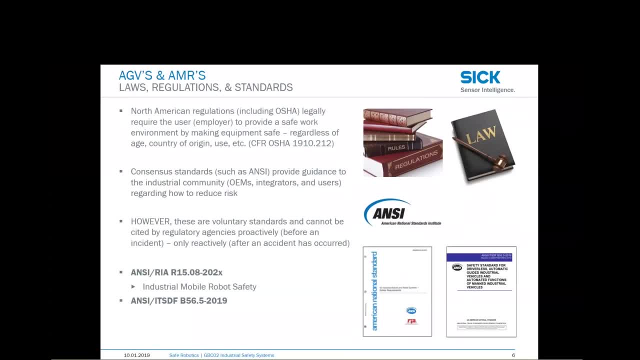 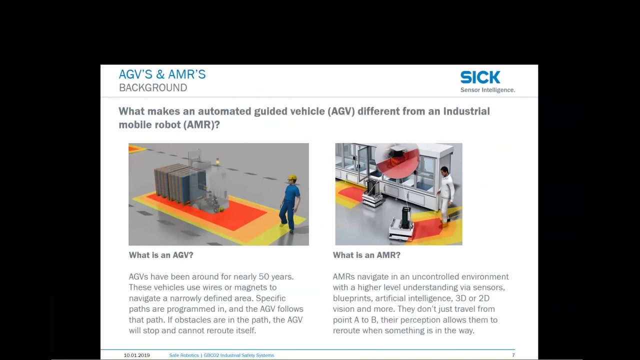 And we'll talk about the newly released ANSI ITSDF, the B56.5.. This is for AGVs- safety standards- automatic industrial guided vehicles- And we will take a look at that standard a little bit and talk about its application. So what makes automated guided vehicles- AGVs- different from industrial mobile robots? 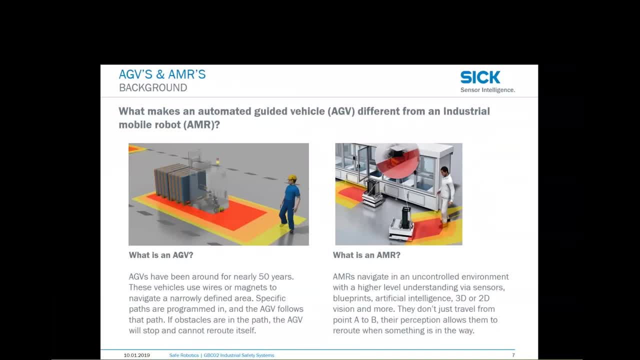 So the main difference is how they follow their path through any given space, right? Most AGVs follow predetermined paths. That means they go from A to B in a predetermined way and they are guided by their navigation system along that path, And AMRs. 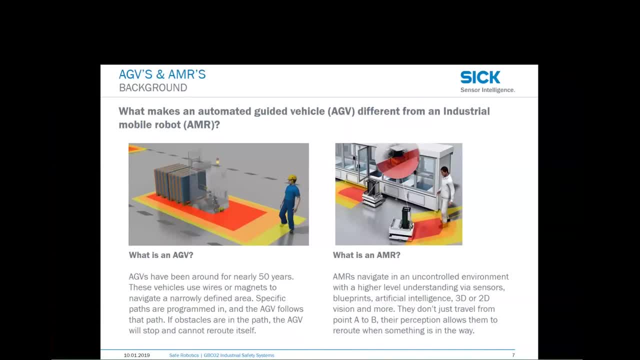 AMRs, on the other hand, are autonomous in nature, which means that they can determine their own path. They can use AI, They can use path planning, They can use other implementations of technology to help them navigate through a facility and therefore can find the most efficient route, considering other influences to the space. 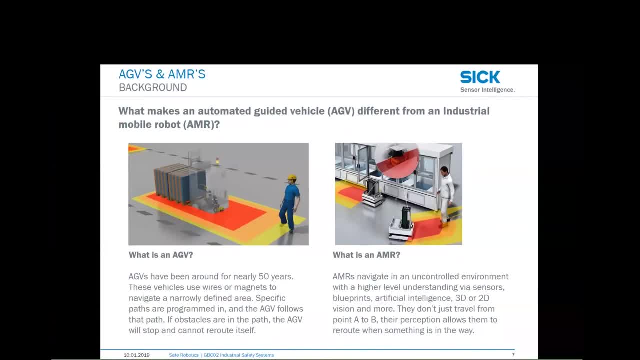 like people or blocked aisleways Or even other AMRs operating in the area. So they'll follow suggested paths, if they exist, but they do have the freedom to find their own way through the facility to get from A to B. So the difference leads to differing methodologies for ensuring safe operation and therefore 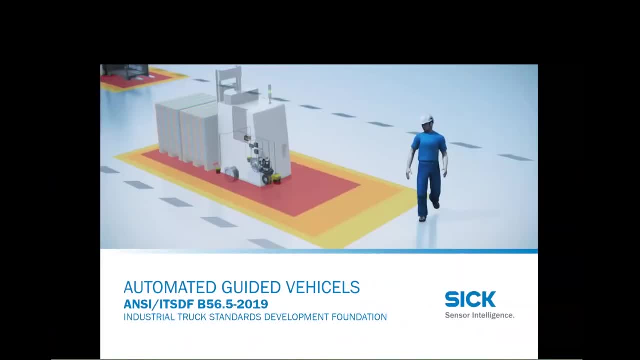 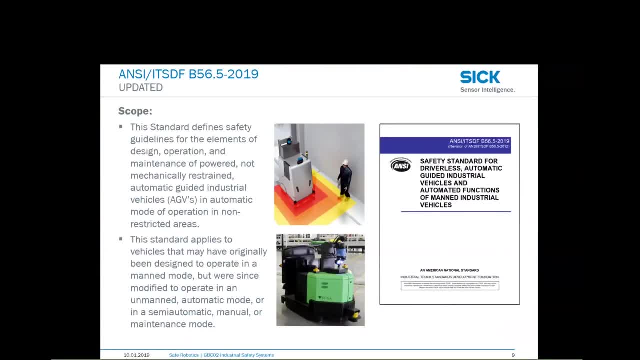 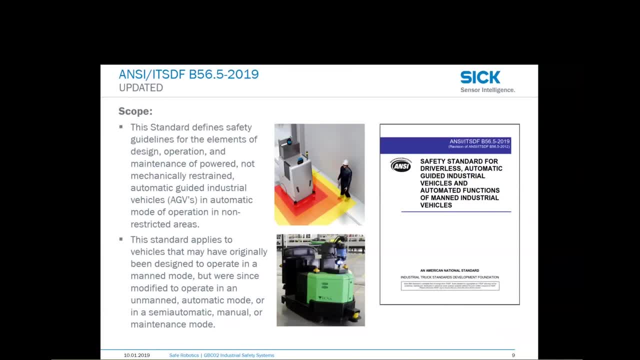 this is found in part two of the standard. or, if you are the system supplier or the manufacturer, you'll find information pertaining to your activities in part three of the standard. The standard does provide for the system. The standard does provide for the safety guidelines for the construction and the implementation. 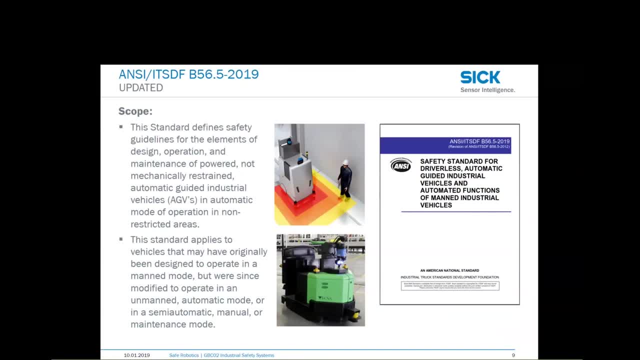 of these AGVs, And also under consideration is manned vehicles that have become unmanned and may be redeployed in a semiautomatic manual mode. So that's also something to consider, but that's the general scope of the B56.5.. 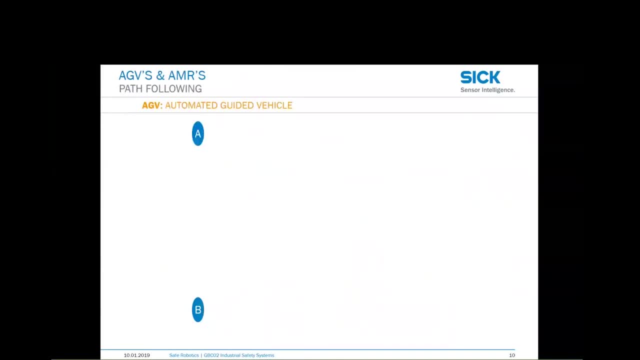 So let's take a little look about path following For AGVs. typically, an AGV again has a predetermined path from A to B. When we look at an autonomous mobile robot, however, it may take a predetermined path, but it may. 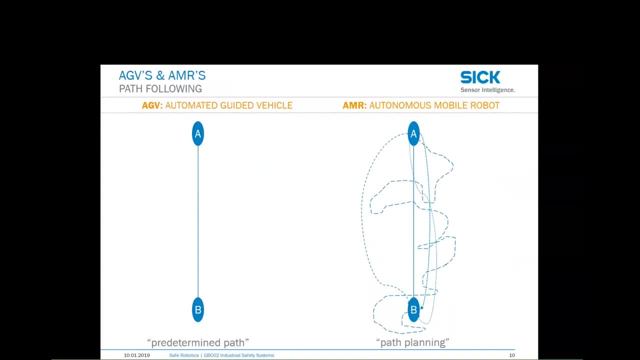 have path planning. It may take other routes to get through the facility from A to B. Therefore, it can leave the predetermined path and find its own way through its navigation An AGV also- when it determines that there is an obstacle within the path, this could. 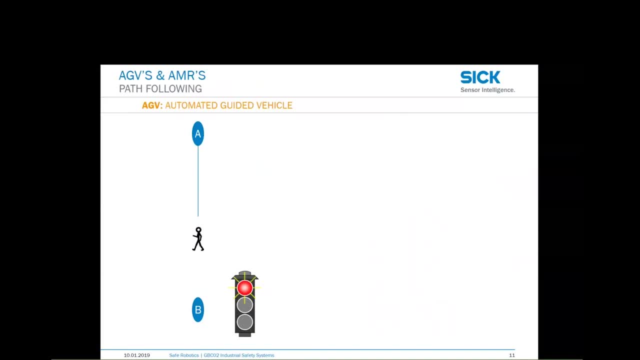 be an object, could be a person. it comes to a halt right. Once the object is removed, it may continue along its path. There are requirements in the standard for how this has to function, how it has to stop, how it has to sense the speeds. 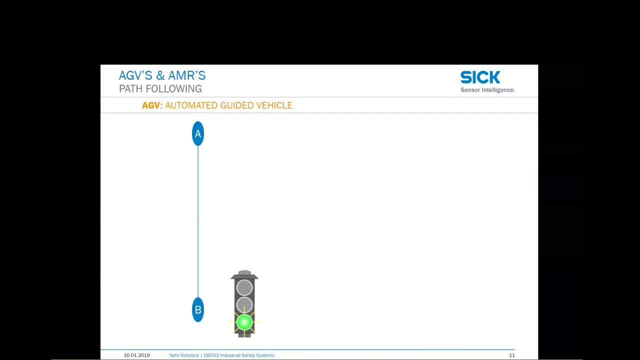 The object detection, The speed, The capabilities of the devices on the platform. This is all covered in the standard on how to go about doing that. Some AGCs or smaller versions and even AGVs can either slow down and then come to a stop. 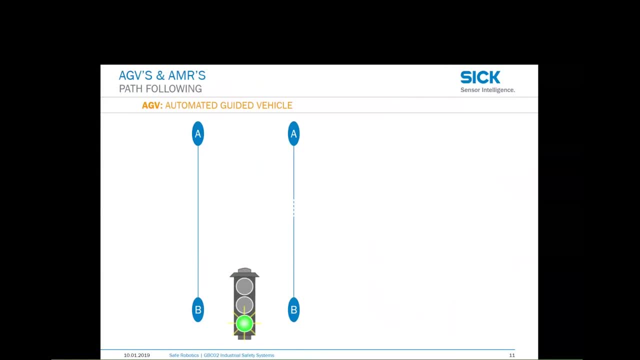 when the object is detected again and move on as necessary. Autonomous mobile robot. however, when it detects an object, it can use its navigational algorithms and facilities to find another path through the plant. This is a typical difference between these types of navigational methodologies found. 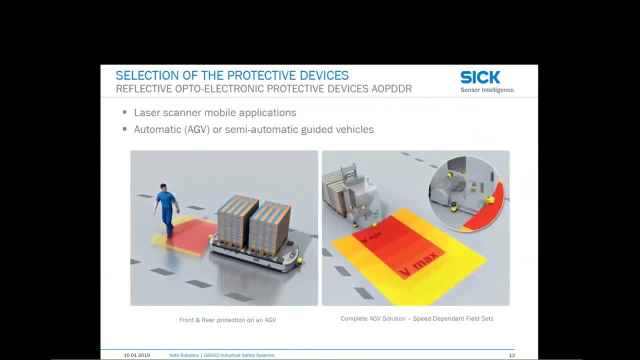 in both platforms. If we look at traditional AGVs, they may be single direction, they may be bidirectional, but they follow a path and therefore they need some sort of object detection capability within that path So that they can determine if there is an obstacle obstructing their way. 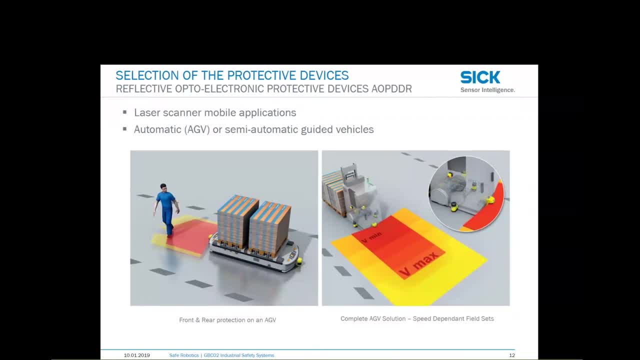 They can change speeds, they can look around corners as they turn following the path And typically 2D LIDAR is a very typical approach to doing this object detection. You can also use bumpers, but there are requirements for using the bumpers and the vehicle still. 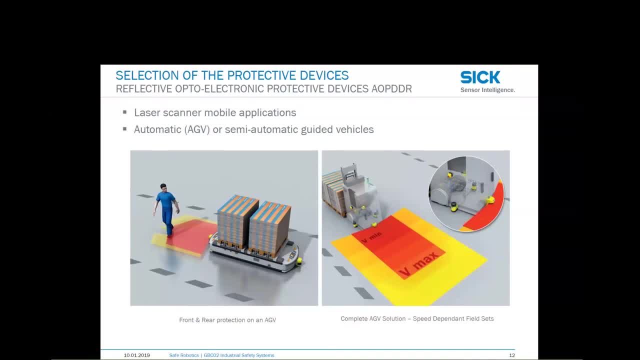 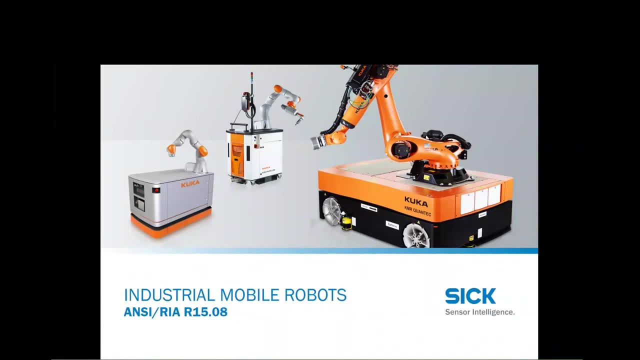 needs to stop, So you can stop in a predetermined way before it comes in contact with the object, even using bumpers. So let's take a look at industrial mobile robots then. This is the RIA-1508.. This is a new work item. 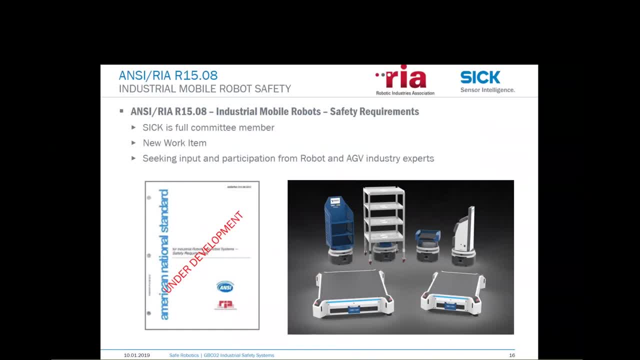 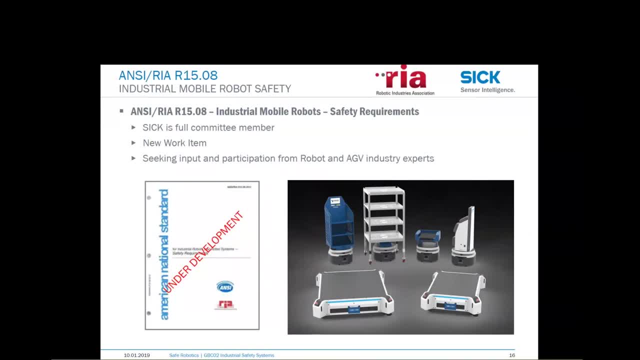 on this committee from both robotic and AGV experts as well as end users. It's always good to have a lot of points of view when ensuring that the standards develop, thinking about all of the technology available as well as tried and true methodologies that come from industry experts who have also worked with the RIA. 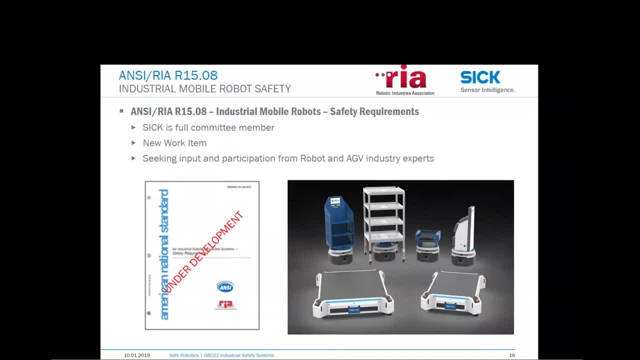 have already worked with these types of platforms in the past, sick as a full committee member we are. we are facilitating and helping to write this standard and i i would suggest, if you are interested, that you get in contact with the ria and see if about joining this committee, if you. 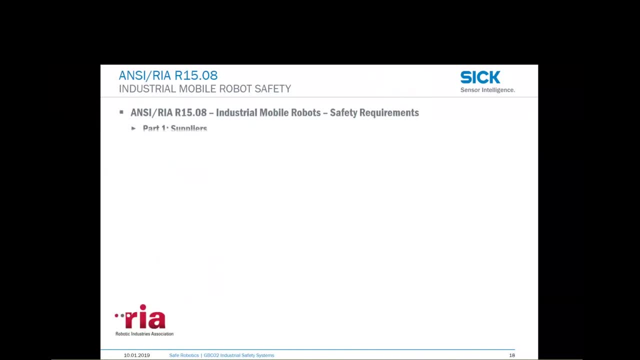 are so interested. currently, as i mentioned, this is under development. so a target release for part one: this will be for suppliers. these will be for manufacturers of these types of mobile robots. so these mobile platforms they still are looking to try to release this next year about mid-year. it is a lot of work. there's a lot going on in really getting a lot. 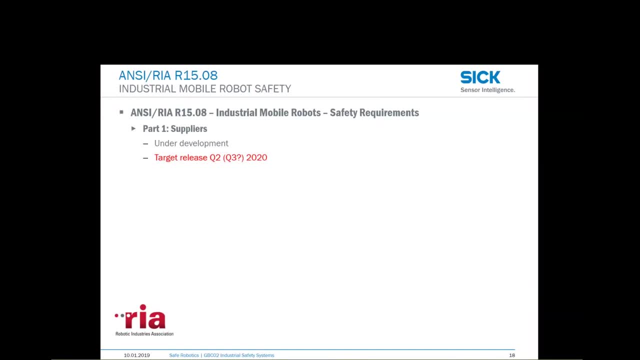 of the definition and the scope for the manufacturers. a lot of these platforms are already being manufactured and therefore there is a lot of industry expertise on on the standard and on the committee who are helping to to implement this and they're bringing a lot of real world uh information and background to to the standard committee. part two is for the 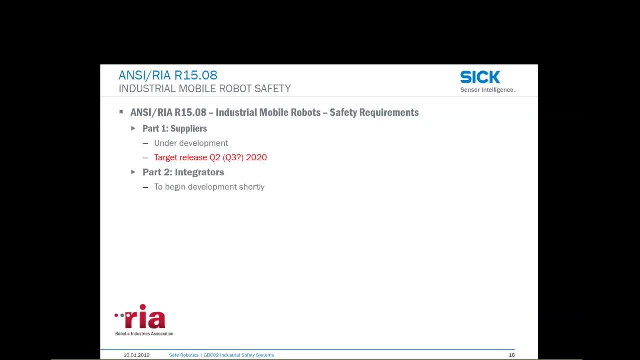 integrators. the integrators um, these will be the organizations and the groups that will be required to implement these devices into the real world applications and uh deploy fleets of these, if you will, and the systems that support the fleets for navigation throughout the facility. that will begin shortly. but the info, but the standard uh writing committee. 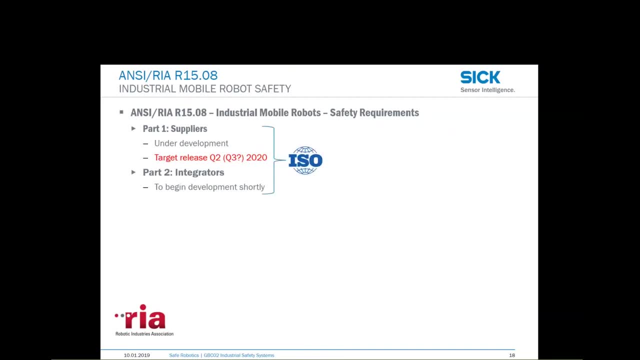 hasn't gotten to that section yet. in the iso world, this is all that's required for a development of the standard um. therefore, end user information will begin development shortly. but because in north america, and specifically in the us, we are an end user, uh, as i mentioned the responsibility, 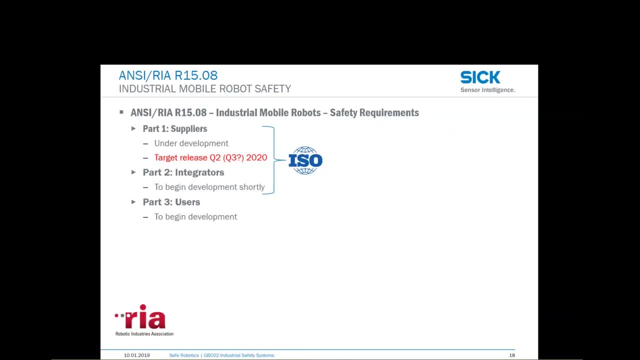 is on the end user. therefore, we need additional information in the standard to support the end user and the safe implementation and overall life cycle management of such systems. so that'll also begin development ongoing issues with defining the scope. we'll go through this in a little bit of. 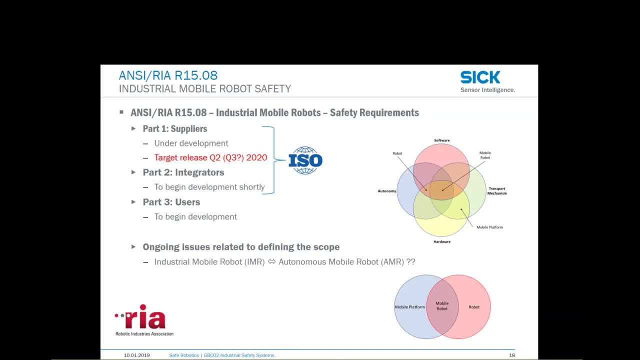 detail here. um, you know, there's a lot more to just saying i have a platform and i'm going to attach something to the top or i have an autonomous platform. there's other things. there's software, there's ai, there's transportation information, there's what is attached to the platform itself. 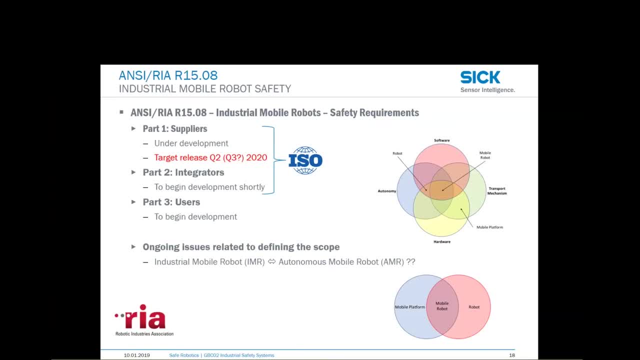 is it a robot? isn't an articulated robot? is it dynamic? is the attachment in motion? do performing automation while the base platform is stationary, or is it moving? these are all very interesting topics that take a lot of thought to think through properly and therefore the standard writing. 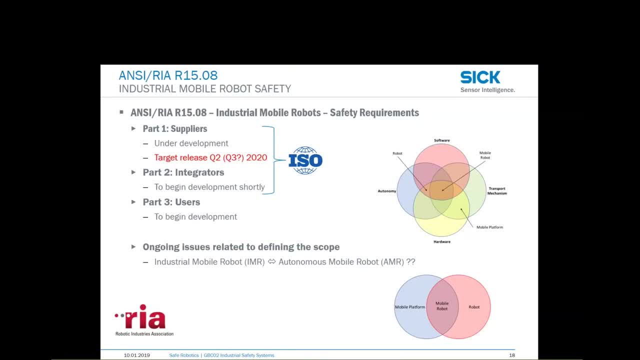 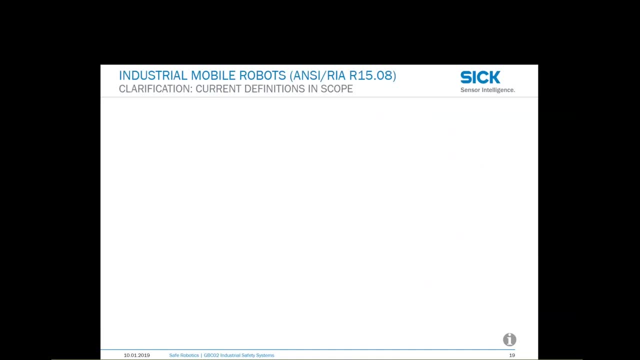 committee is struggling and wrestling with these uh, these uh topics as we speak, right, so let's take a look at the current definitions of the scope of this document. i think this is really important when talking about the requirements for industrial mobile space. like you know, the standard writing code for the first five months. the key word here is: 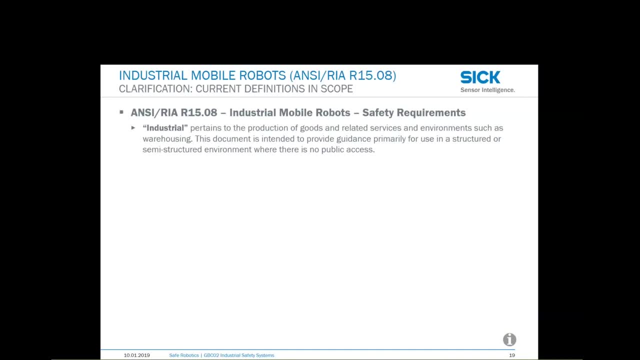 industrial. these are being the standard is being developed to give guidance to industrial applications, not in the public space. we expect these vehicles platforms to operate within spaces in an industrial environment where most of the people they come in contact with are trained. they understand the operation of the systems and the platforms within the industrial space. 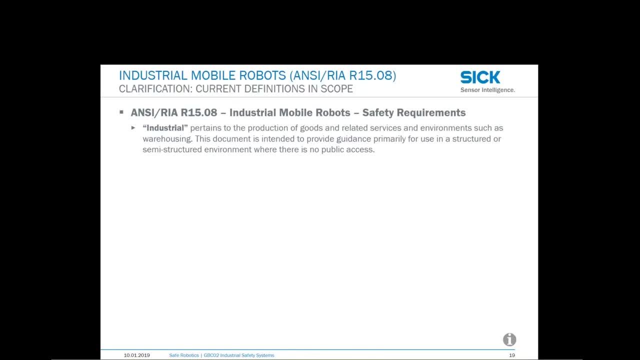 Therefore, certain risks and certain tasks and hazards are more appropriate for this type of application. No public access Mobile. Now, this does refer to ground-based mobility and not to water or airborne type of vehicles. So if it's mounted on rails, if it's in water or it's airborne, it will not be covered by 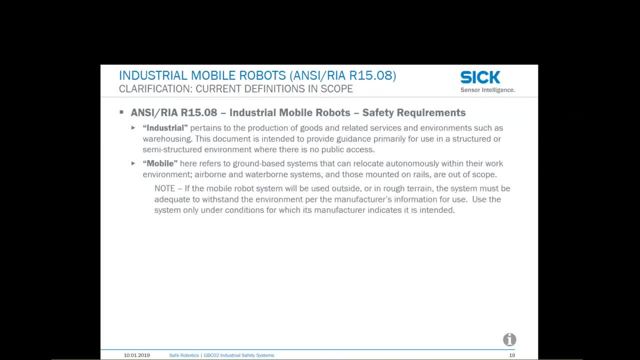 this standard. However, if it's mobile in an outdoor application, there will be some additional environmental requirements that will have to be considered both by the manufacturer, designer, implementer of a platform or mobile robot, as well as the integrator or the application for its. 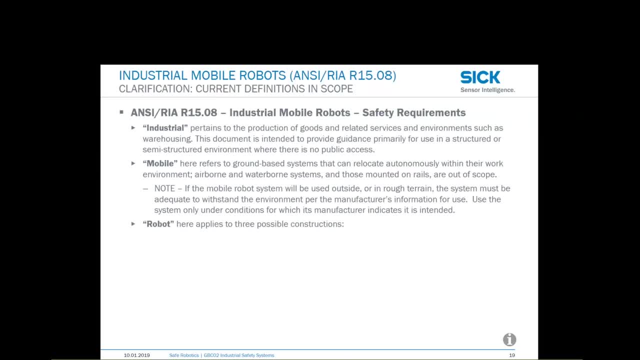 intended use. The robot as we talk about the platform actually applies to several different applications, Three possible constructions, and we'll talk about these in detail. but it could be the industrial manipulator attached to a mobile base, which may or may not be autonomous. 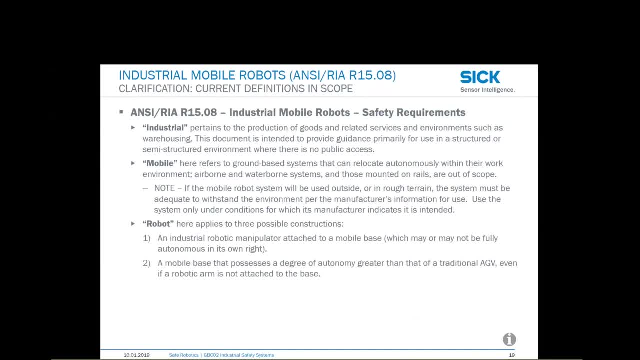 the mobile base that has a degree of autonomy greater than your traditional AGV, with or without anything attached to the base. and then the same unit with the mobile base and a robotic articulated arm with a degree of autonomy, and is capable of operating dynamically. 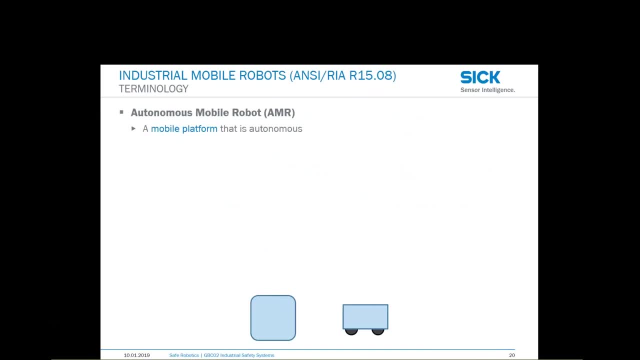 So let's take a look at some of the terminology that's being defined underneath the development of the standard. So, as I mentioned, an autonomous mobile robot is a mobile platform that is autonomous. That means it has the ability to navigate using obstacle avoidance trajectory plans. 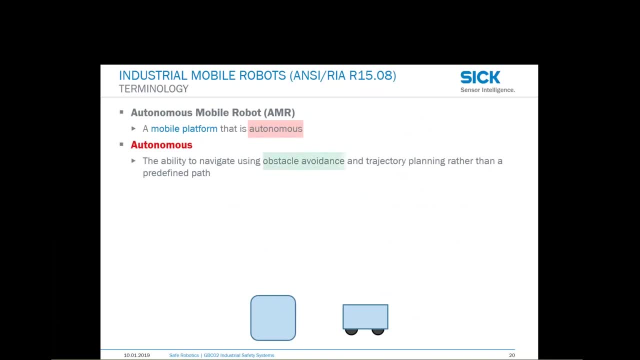 trajectory planning rather than a predefined path. So what is obstacle avoidance? So preventing interference, such as approach contact with objects, whether it's a fixed object or a moving object, like other AMRs and or persons in the area, detecting them with sensors and adjusting their trajectory. 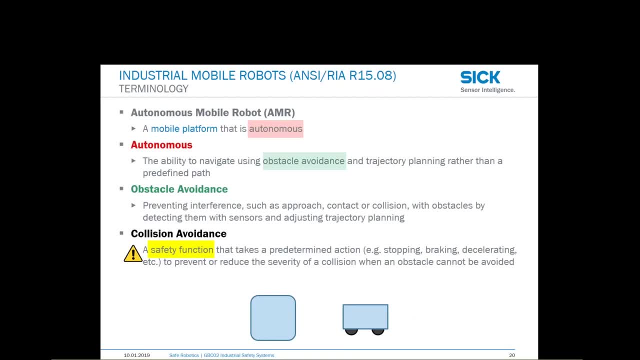 So collision avoidance, then, is a safety function, Right, So we're reducing risk with this application. So the safety functions take a predetermined action. Do I slow down, Do I stop, Do I take another path, Do I steer around to avoid collision? 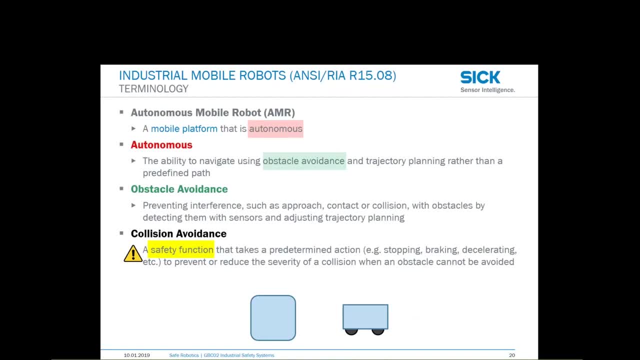 Right, This is a safety function. Therefore, it relies on the safe operation of the control system and the sensors giving the sensory input to the object detection. So there will be requirements around The safety functions and the implementation of the safety functions on a platform. 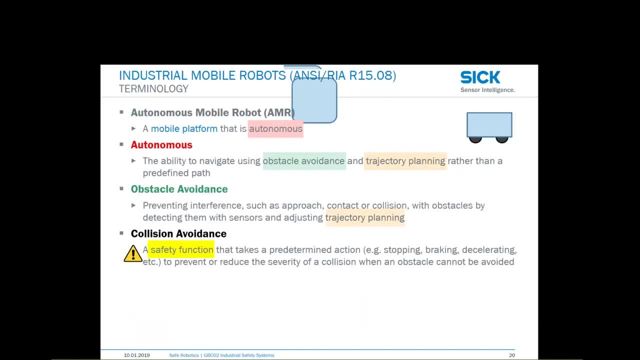 The trajectory planning right. So again, trajectory planning is about planning the path with time as the parameter. How do I get from A to B? What's the quickest way to get from A to B, where I avoid obstacles and therefore can be the most productive and efficient in moving through the facility? 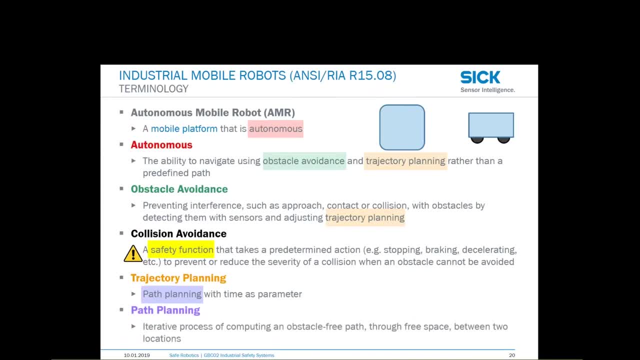 Now, path planning is this iterative process of using different ways of computing an obstacle-free path. This can be AI-supported, cloud-based, could be map-based. also, information taken from other AMRs operating in the same facility. This is a fleet, if you will, and fleet management throughout the space between any two locations. 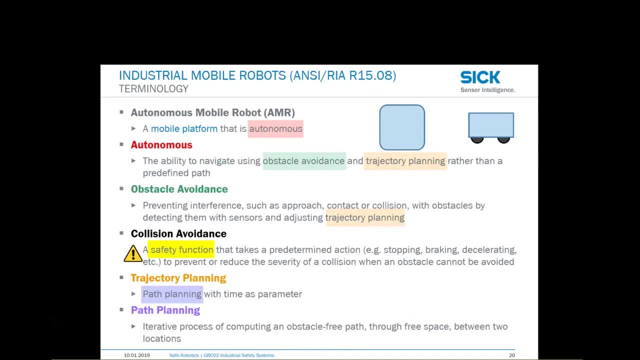 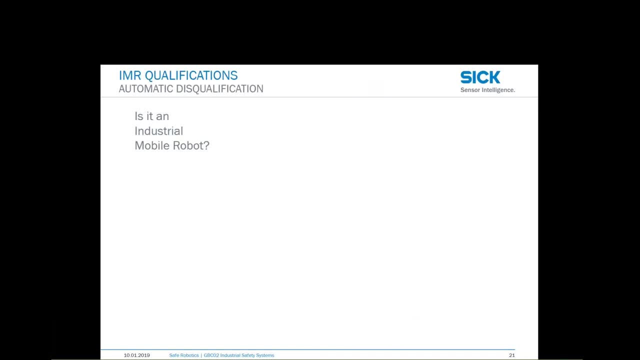 that any given platform needs to navigate in. So let's take a look about the qualifications of the standard, as it addresses the different types of AMRs that will be covered and won't be covered by the standard. So if we think about, is this an industrial application? as I mentioned the standard, 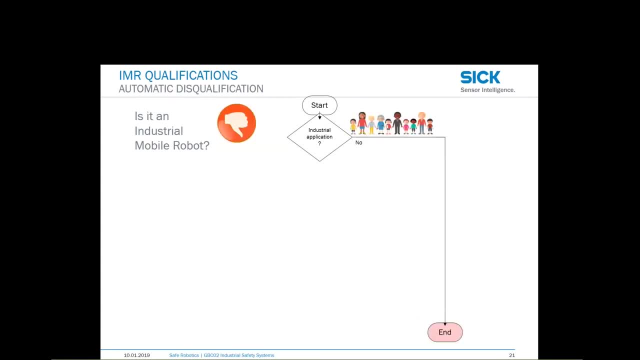 is governing industrial. So if this is a public space, this standard will not be applicable If it is a mobile platform. if it isn't a mobile platform and it's stationary, okay, then it has a manipulator of three or more axes. 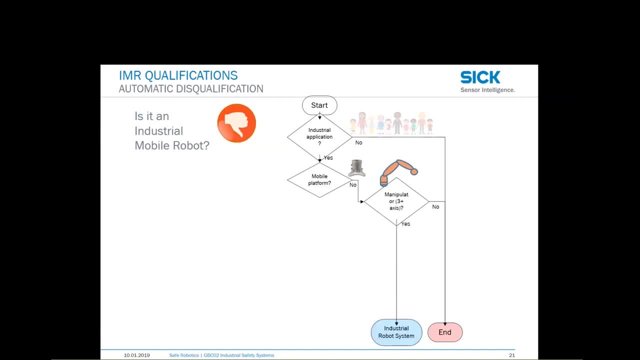 Well, we know that there's a standard for that, and if it is, then that's an industrial robot system That's covered under the R-1506, so it will not be covered by this standard. If it does have navigation, but it's manual and it does not have a manipulator, then 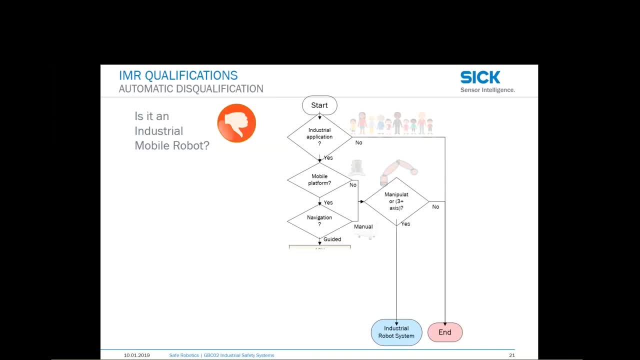 it won't be covered. However, if it is guided as an AGV, okay, it is a mobile platform, but, again, if it doesn't have an attachment, then this is covered by the AGV standard. So it is a guided vehicle. 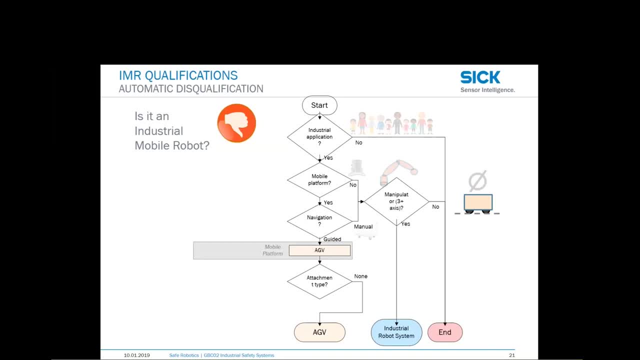 We have a standard for that. We know that's the B-56.5, so we're covered If it has some other type of attachment as well. potentially, regardless of the attachment, if it's still guided, it's still AGV. 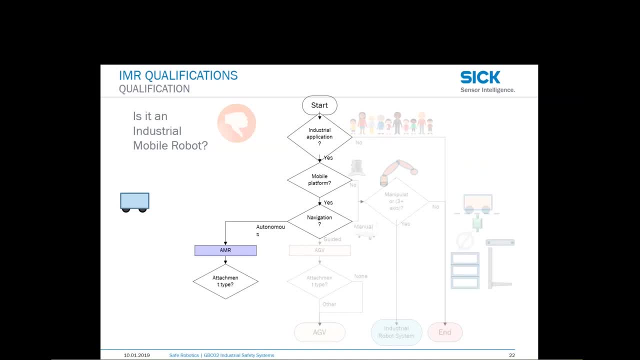 If the navigation, however, is autonomous, it is an AMR, an autonomous mobile robot. But let's take a look at that. Okay, Let's take a look at the different types of attachments. If we have no attachment, this is a Type A. So the standard is defining the requirements. 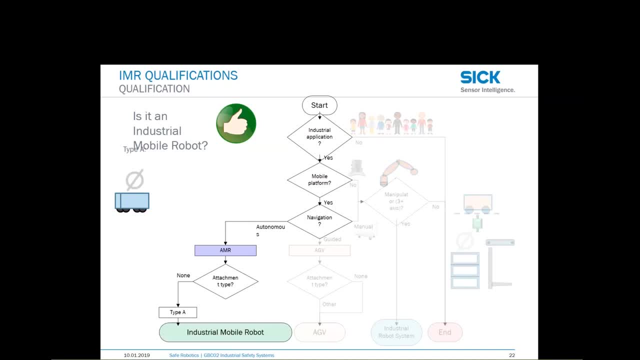 for a Type A mobile platform. If it has another type of attachment, this is a Type B industrial mobile robot. Could be a conveyor, could be bins, could be a cart, Could be a fork lift. If it, however, has a three-plus-axis mobile manipulator, this will be considered a Type 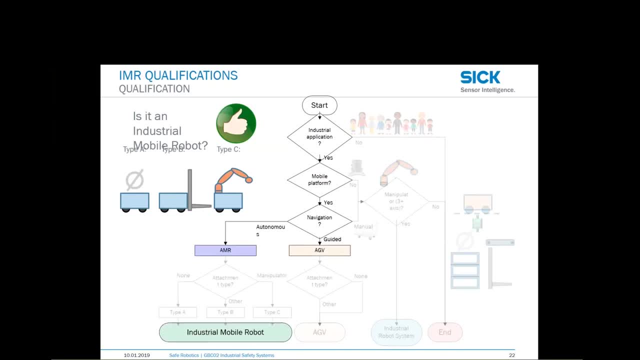 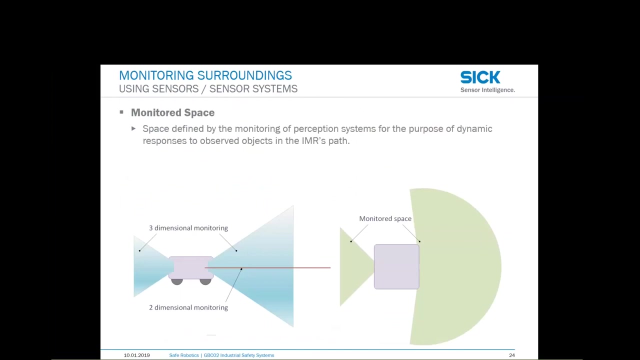 C. If we have a guided vehicle mobile platform and we have an attachment type as a manipulator, this will also be considered by the standard as a Type C mobile manipulator. When we think about monitoring for these types of platforms, we need to think about: 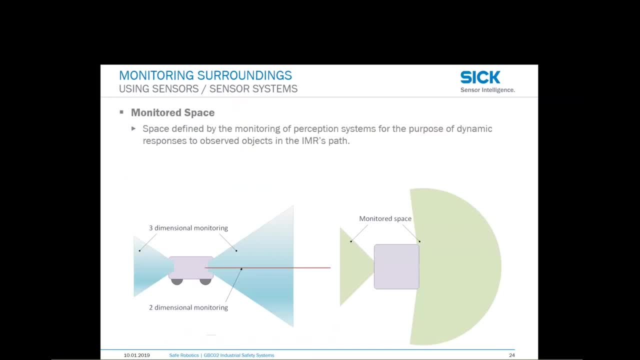 monitored space. These units are moving and they're going to add some dynamic, potentially add some dynamic applications. Again, as I mentioned, we have to think about – traditionally AGVs have thought about- 2D space. just need to see the line of sight and the direction of travel to ensure obstacles. 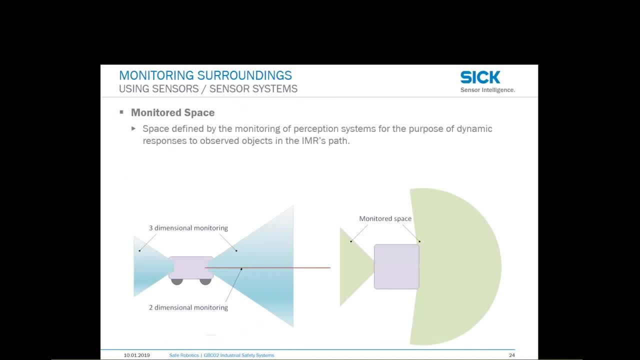 are detected and that they're not impacted, or we have the collision avoidance with objects Once we start to put manipulators and other types of attachments to the tops of these platforms. we now have to consider a potential 3D space, things above the line of sight, or 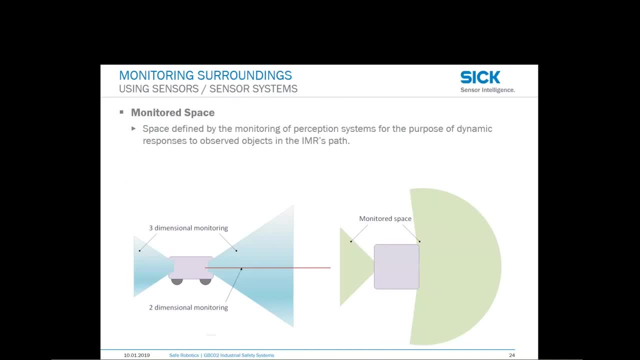 the detection at the floor level, At the floor level, of objects in the path of travel. So we have to think about that space and the 2D space. Now the monitoring system consists of components that are not necessarily safety rated. There will be requirements in the standard to address the level of safety required based 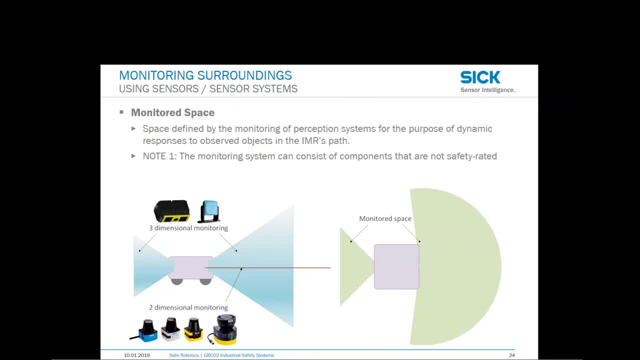 on the risk. This is what the risk assessment will help you define. and again, there is a new standard- WC62998, that allows you to implement sensors and safe applications. If you're interested, you should take a look at the standards, the newly published standard. 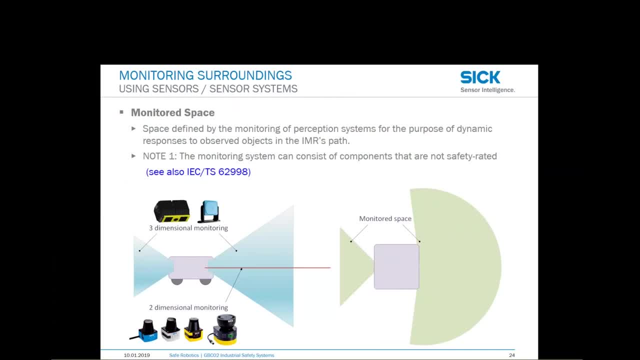 and it gives guidance for safety-related sensor systems specifically for these types of applications. The monitored space: when it can change dynamically, we need to think about again things going on at different types of applications. Again, this is a new standard. 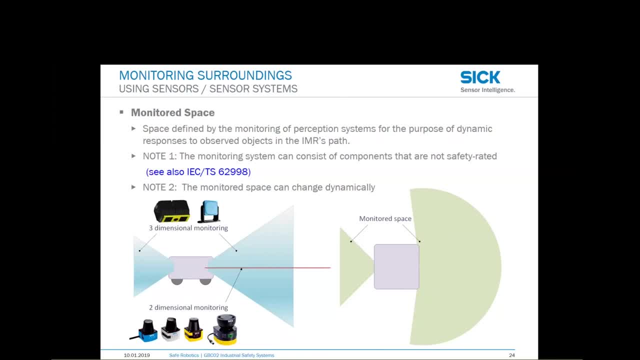 There may be different types of applications, but what this means is we can need to observe that the orders want to be received when it's in motion or object 언 manufacture. This means when the order is laying around that. what is the change that we have to do? 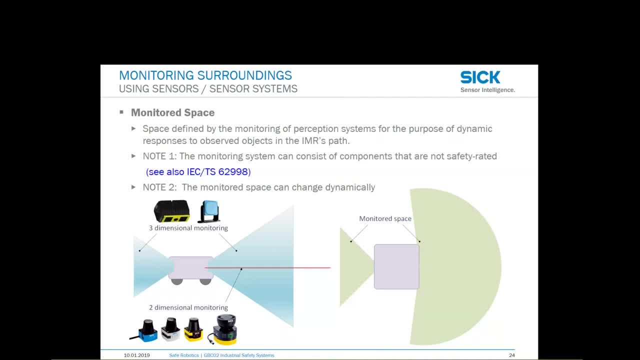 in order for that to happen, for safety reasons, Sometimes down the line. if it gets too high, if it goes too low or if it chooses off too low, the alert goes off too. give the machine a chance to gesture in the direction this. 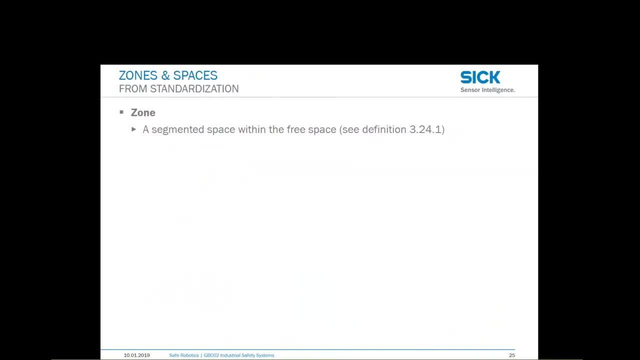 object is being directed. Yeah, and I will say I'm going to take multiple samples and I think I'll try to make some ары as much progress as possible, as it's starting to develop scope around the space. so if we think about in the AGV standard, 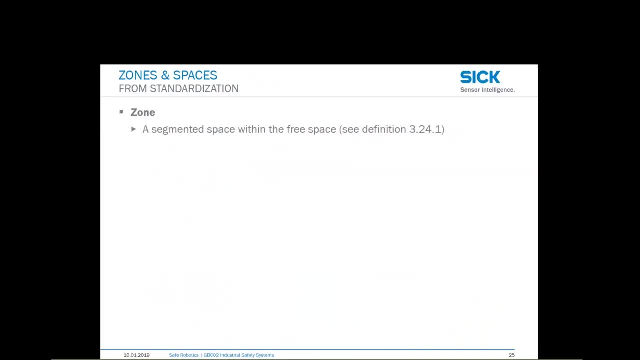 it covers the space- restricted space and operating space- and it has all the requirements defined in the standard, which is very well thought out and traditionally has been understood very clearly, about how to define clearances between immovable objects and the path of the AGV, and so on and so. 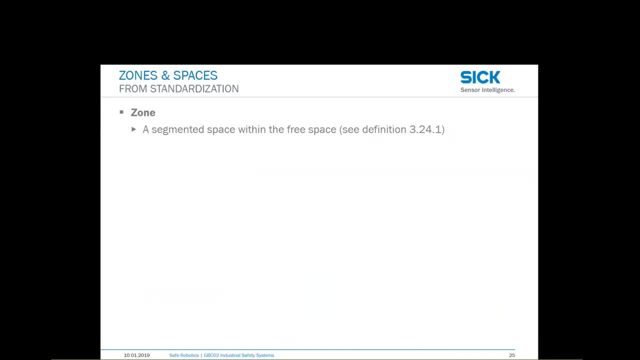 forth thinking. well, taking that thinking that's been available to us for for quite a few years, as in the AGV world. now we have these more dynamic, autonomous platforms. so how will they know about these clearances to other objects and be able to stop and ensure safe? 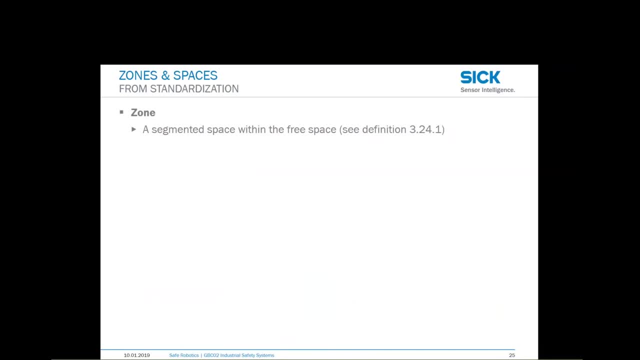 space is allowed for for safe interaction with humans or other other personnel and or objects within the space. so, thinking through this, the standardization committee has started to define some of these methodologies for thinking about the operating space that these platforms will run. a segmented space within the free space is a zone. 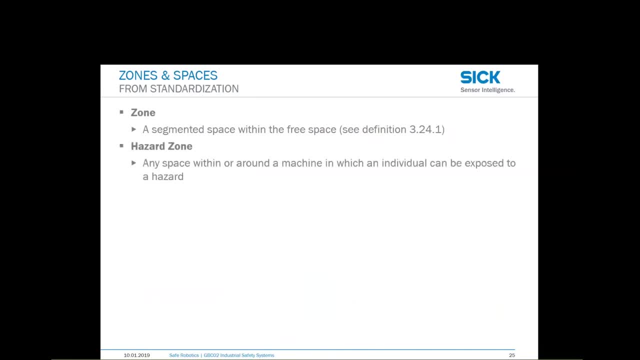 right, we'll have hazard zones. these are spaces in and around the machine which, in an individual, can be exposed to a hazard, so it makes sense if you're in this area, there are hazards associated with being in this area. for an IMR, this will include all the spaces of inadequate clearance. 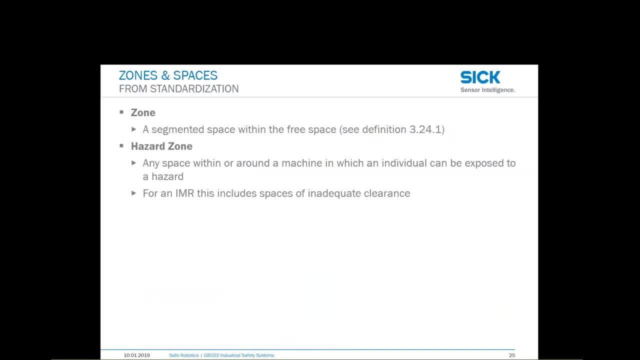 as I mentioned, there are clearance requirements and the AGV standard. some of those same clearance requirements, I'm sure, will find its way into the standard and there will be minimums of clearance around hazards. some of those will be defined as keep out zones right a zone excluded from the free space um free space också有 ור呢這個環境將解決這個 izer filled area within the distance of the free space um free space, en comparation to all the원 않은Phasein. 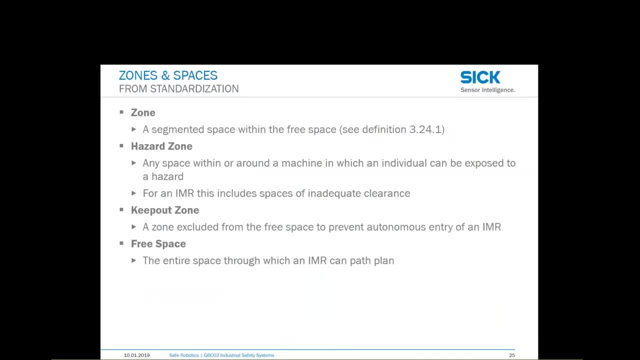 be allowed, which an IMR can pass plan freely. There are not expected to be any fixed objects. There may be some dynamic objects or other movements in the area, but in this free space the IMR is free to navigate, But once it goes into an area where it's absolutely restricted, 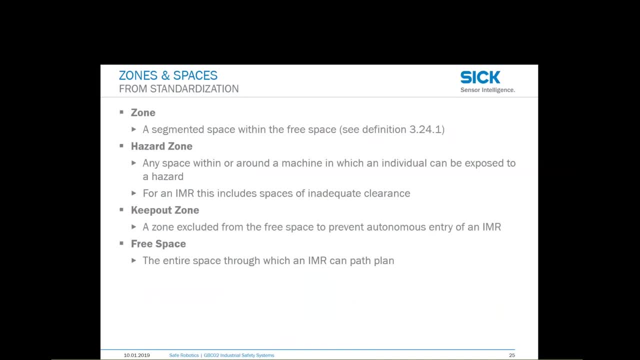 these will be keep-out zones. There just won't be enough clearance. It's already been predetermined. There's no need for the IMR or the AMR to move into the space, So this will be defined as keep-out spaces, keep-out zones, And that brings us to base footprint. So 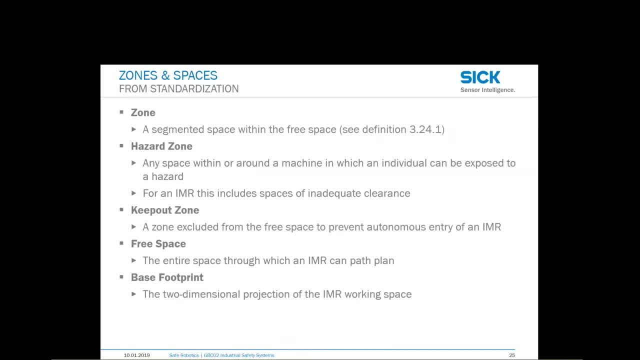 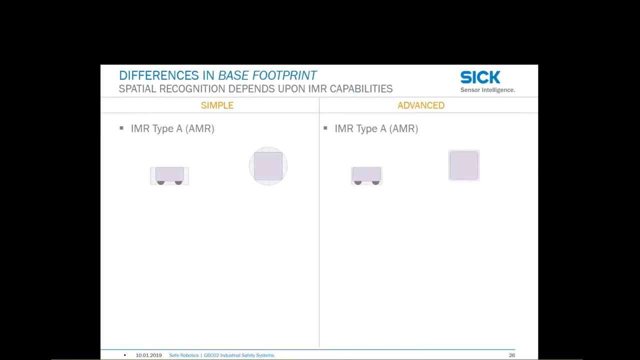 the two-dimensional projection of the IMR in the working space will become its base footprint. So what is special or what do we need to consider when we think about the base footprint? So, when we think about the IMR type A, just the mobile platform, a simple or smart? 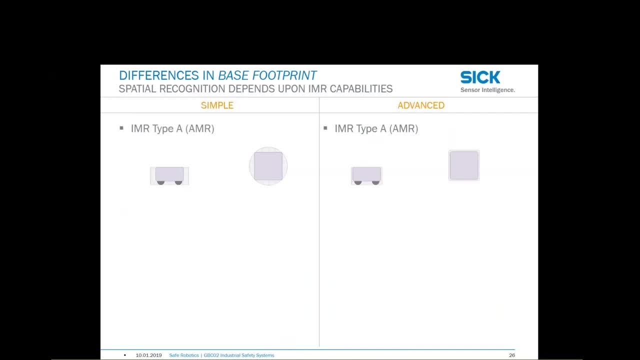 implementation or, if you will, a non-smart implementation- really can navigate and can object detect. But this is like your Roomba, you know, eye vacuum running around. It really doesn't have a good picture of what it sees or what the space is, It's just bumping its way around. 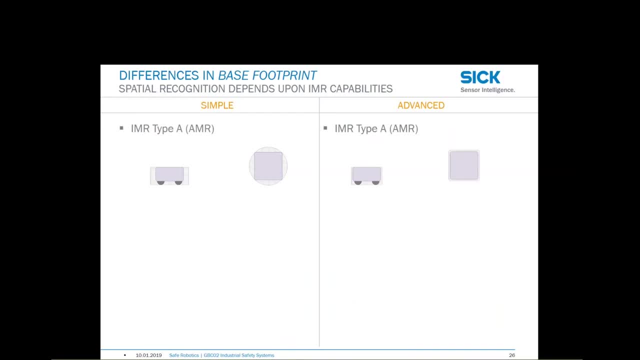 And therefore needs a little bit more space around it, because it's really not navigating with any exactness. It is just operating in free space, has safe algorithms to do that, but it's going to need a little bit more footprint. However, a type A IMR. 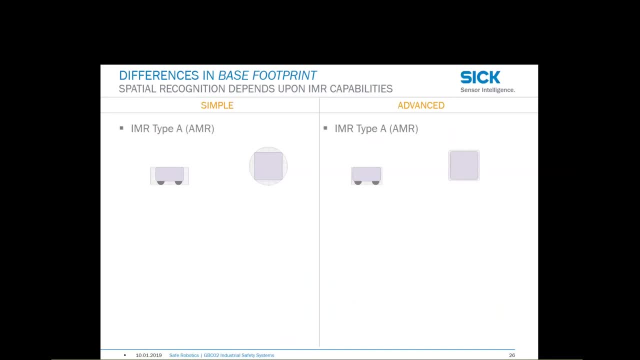 which is more advanced, is going to have advanced navigation. It's going to have more information about its space that it's operating in. This could be a map. This could be a location where it's operating. This could be a location where it's operating. It could be a. 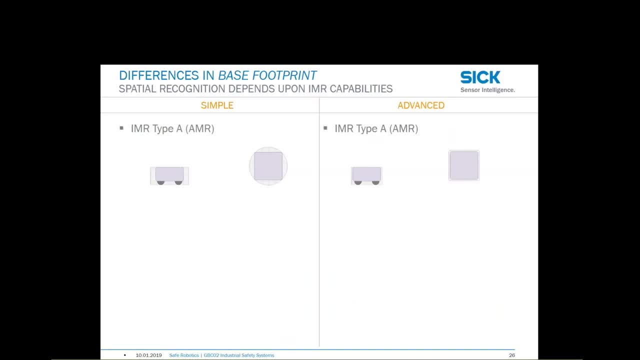 location where it's operating. This could be a location where it's operating, But if you have a type C and you're going to have un-determined or memorized locations of objects or combinations of those, this is. this allows the device to have a little bit more understanding about those. 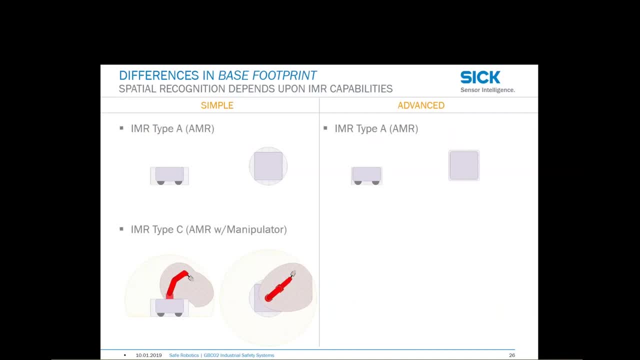 restricted areas around it. So if we have a type C with the manipulator, you can quickly understand that if I'm not navigating in a really defined, really well understood space, I'm going to need more room that the clearances around the manipulator are going to be sufficient. 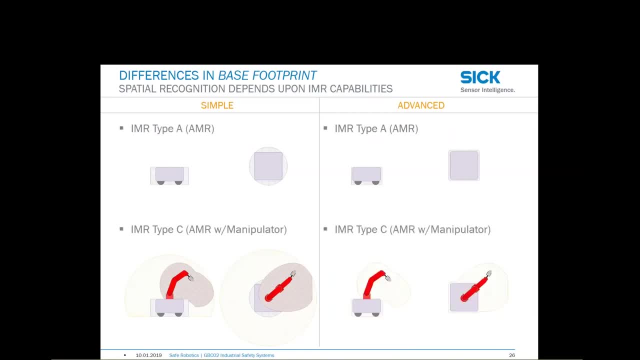 enough to operate safely If I'm going to have a more advanced and I understand where I'm operating. I have these maps, I have this extra information and I have more navigational ability. I can now also understand the safe operational space or 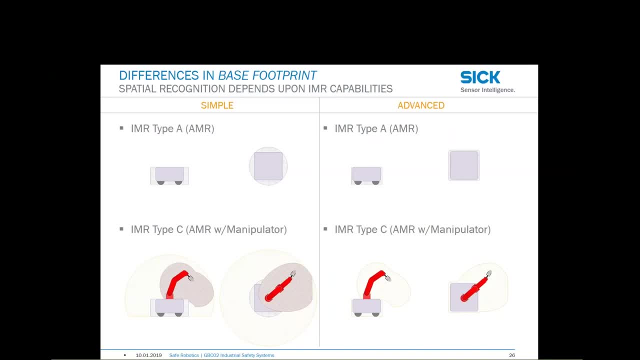 restricted space, if you will, for the manipulator to ensure that it operates safely, Whether that's dynamic or it's fixed. if the platform's fixed and the manipulator is moving, I can then only concern myself with that actual movement of the manipulator while the platform's fixed. But again, the more 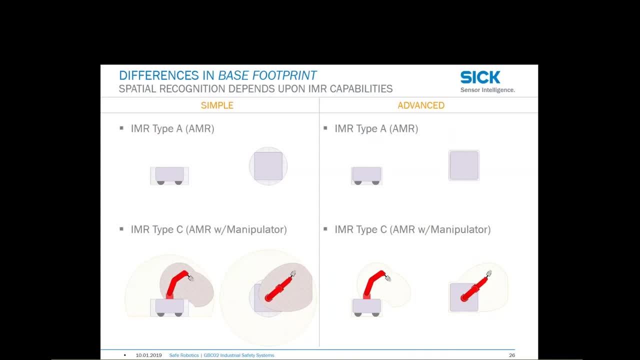 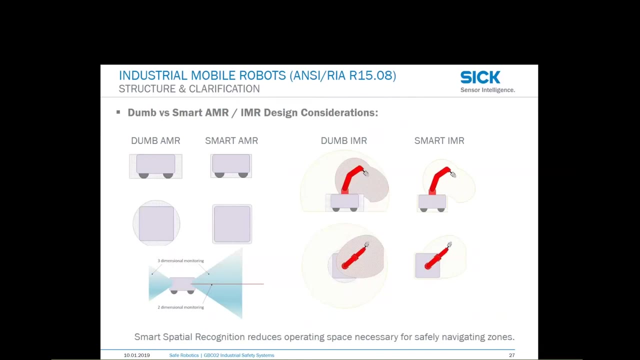 advanced detection capabilities of the platform will give it a little more leeway in how much clearance is required. So in the end, that's a design consideration when we think about dumb versus smart, if you will, So that smart spatial recognition and understanding. 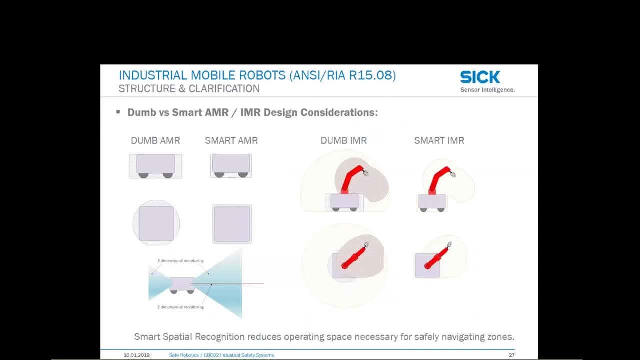 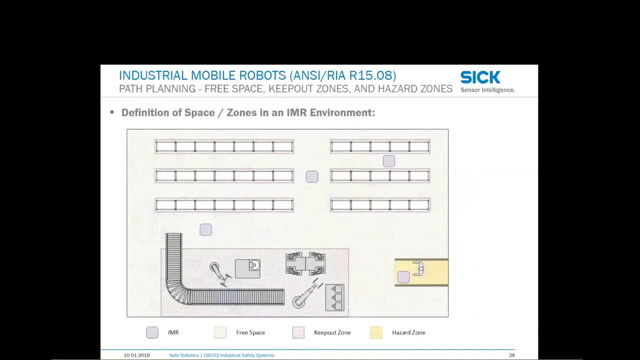 what's in the space is necessary for safe navigation throughout these zones. So when we think about the zones, right, the definition of the space, it might be something that looks like this. So if I'm going to have a more advanced 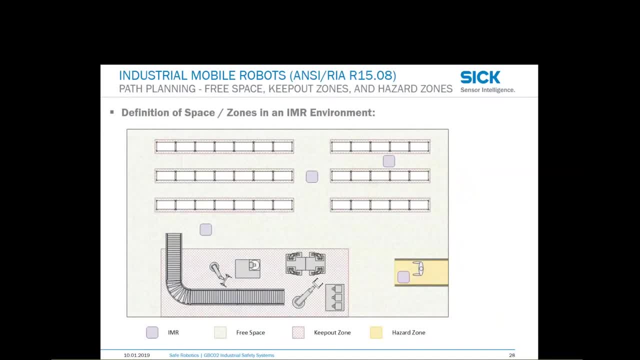 definition of the space. it might be something that looks like this: This is something that gives definition to the free space. you see here in the green, This is the space where the IMR is free to navigate within its autonomy and its algorithms for navigation, Whether that's AI, it's cloud-based, it's map-based. 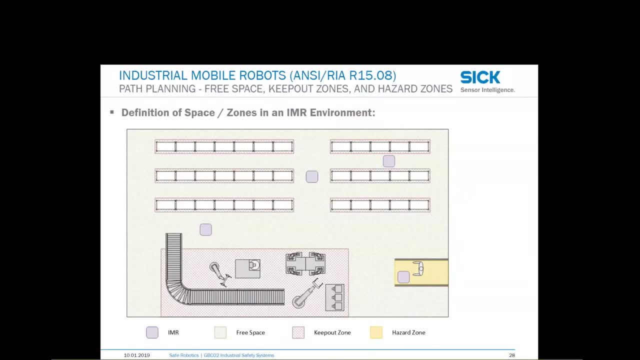 learning regardless. this is the free space that it is allowed to operate in The keep-out zone. this will be areas of other automation or other areas of the facility that are off-limits and there's no reason for the IMRs to operate. 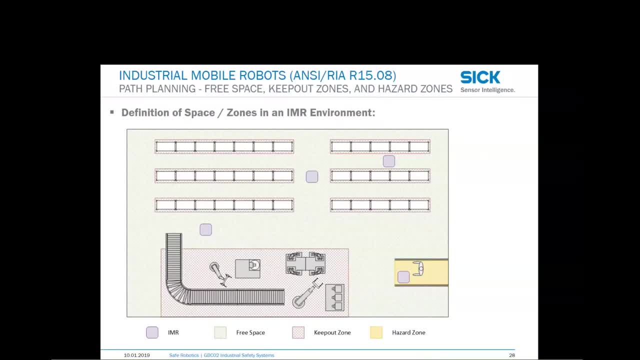 in these spaces so these can be defined and restricted. Hazard zones then are when the IMR may contact other objects, both other AMRs and or objects such as people, and there's some sort of restriction, and that restriction has to be thought of a little differently, because maybe it's a lack of egress. 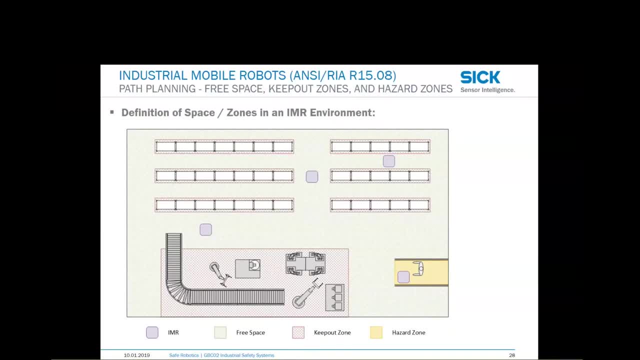 Maybe it's a storage area where the AMR is either retrieving loads or other trucks or other picking up material, dropping off material, interfacing to a conveyor, wherever there might be some interaction, where there will be some space, spatial requirement for ensuring that people are not injured in these areas. 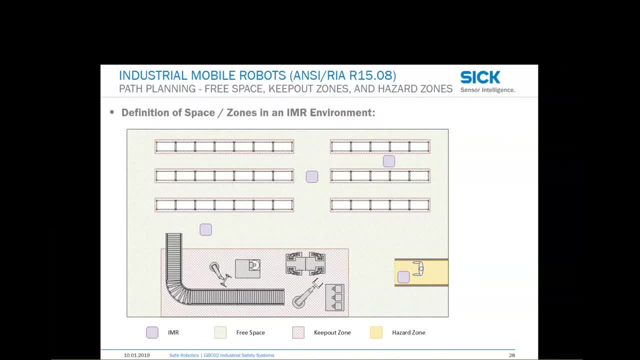 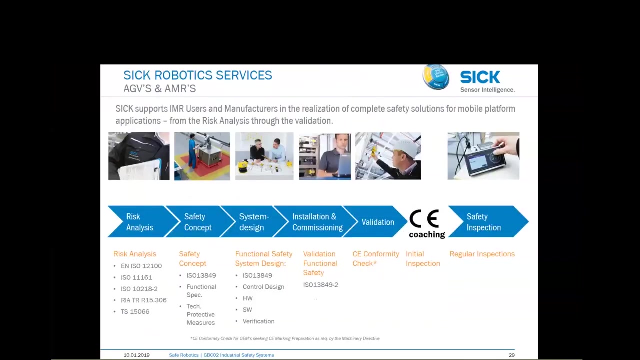 So these are the areas where they may come in contact and there will be some sort of space restriction. So this is the type of environment planning and definitions of the scope that's ongoing within the standard. So, lastly, a little bit about SICK. 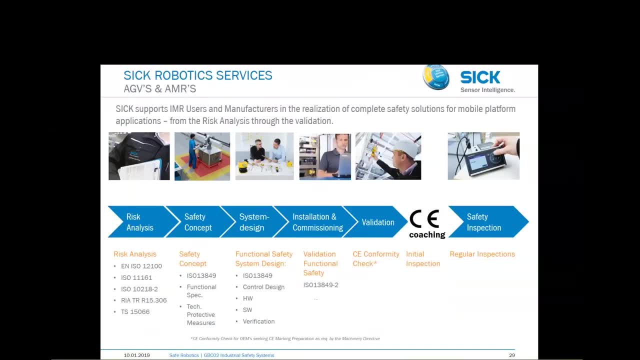 We provide these. as I mentioned, there's six steps that we follow in a logical path whenever we're providing our consulting services and we're thinking about supporting our customers and the application of the sensing products and or their SICK implementation on these types of platforms.